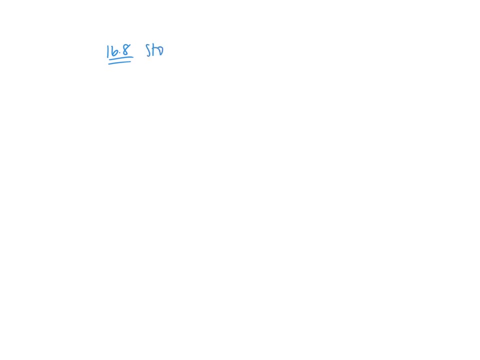 Okay, so section 16.8 is going to cover what is called Stokes' Theorem, And then section 16.9, which is the last section we will do- covers what's called the Divergence Theorem. So all we're talking about today is what's called Stokes' Theorem- Stokes' Theorem. 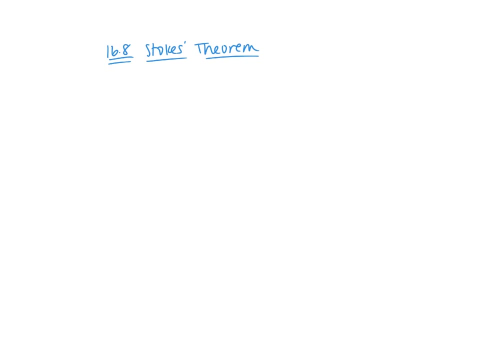 should remind you a little bit of Green's Theorem. So if we're going to start with Green's Theorem, if you recall, that symbol is a line integral that is closed with positive orientation, And if we were taking that line integral of f, dot, dr, which is work, Green's Theorem tells us: 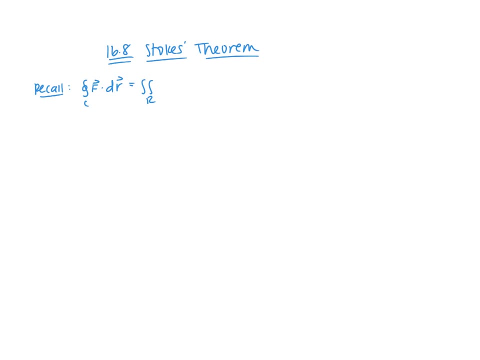 that we can change this into a double integral over the region r of partial of q with respect to x, subtract partial of p with respect to y da. So, if you remember, this is Green's Theorem, Green's Theorem, we have to have a closed curve. 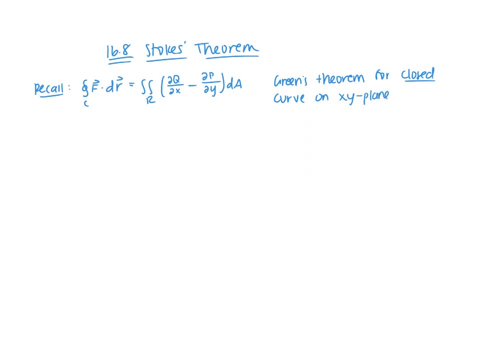 And that curve is on the xy plane. So, if you remember, both q and p are functions of x and y, And this symbol means that we have a line integral with positive orientation. Okay, so one thing that we talked about when we did Green's Theorem. 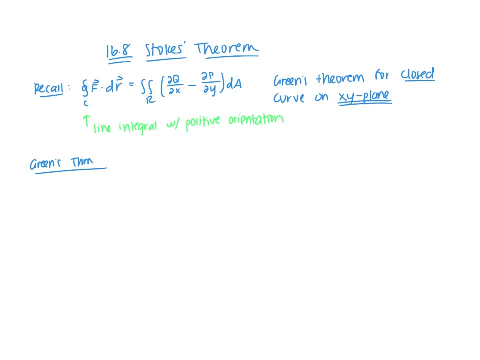 well, it was actually the section after Green's Theorem. we talked about how you can take that f dot dr or Green's Theorem and you can actually write that as a double integral. That involves curl, So curl of f dot k da. 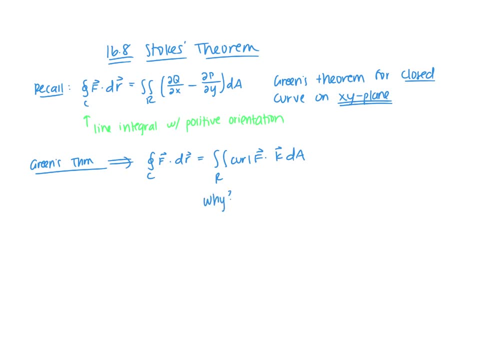 And so, as a quick review, the question was: why are we allowed to do that? So, if we start by finding curl of f, we are crossing the gradient, So partial with respect to x, partial with respect to y and partial with respect to z. 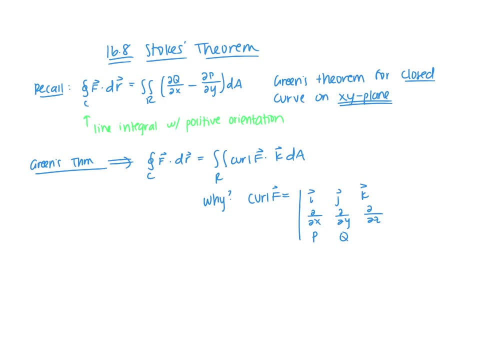 with f, which is p, q, 0.. Remember again: p is a function of x and y, q is a function of x and y, And then we're on the xy plane, so there is no k component. Okay, so, finding our i, 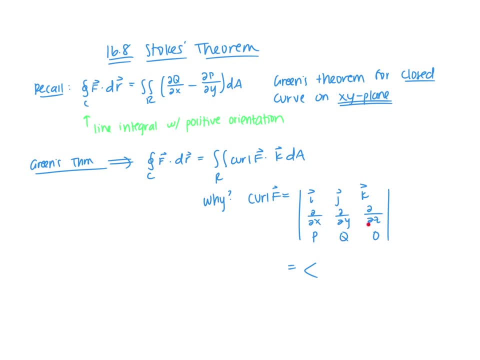 we get the partial of y with respect to 0,, which is just 0.. Partial with respect to y, which is just 0.. Partial with respect to z of q. q is a function, though, of x and y, So there is no z, so that gives us 0. 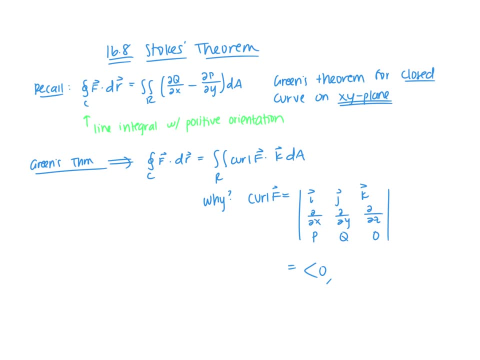 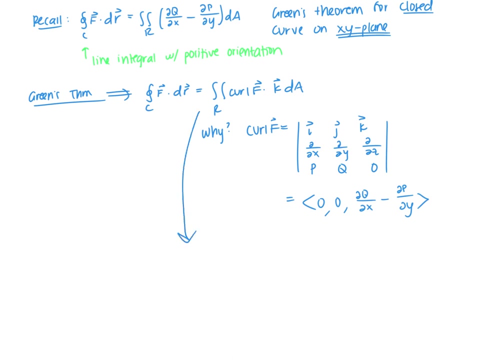 Same idea: for j, we get 0 minus again 0.. And then, for k, we get the partial of q with respect to x. So subtract the partial of p with respect to y. Okay, So then what we're doing is we are taking that curl. 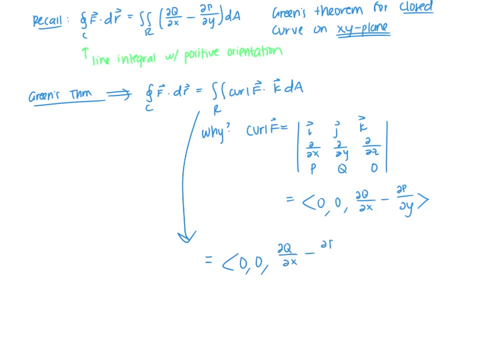 which we just found and we are dotting it with k, and k is 0, 0,, 1.. And you should see, that gives us our green theorem from above. So that gives us the green theorem from above. it's just written in a different manner. 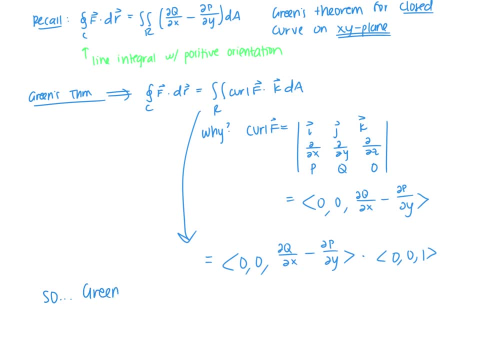 So what that's leading us to is that Green's theorem can be tied to curl Now. Green's theorem, though, like we said above, only works for a curve that is on the xy plane. So what do we do if we have a curve that is not on the xy plane? 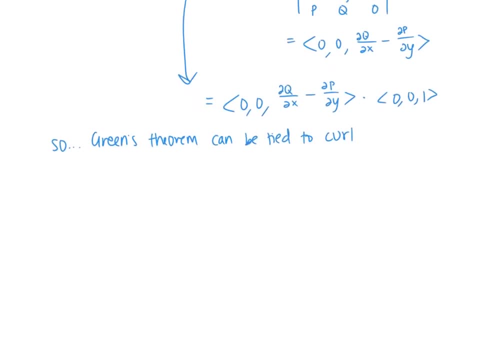 That's what we're going to look at now. So what's new today is we are looking at a similar idea, but in 3-space. So let's say that we have some type of figure like this And it's moving that way. 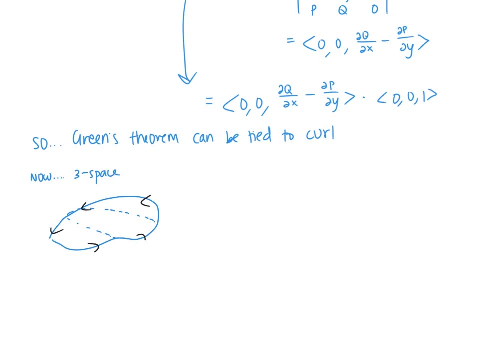 So with Green's theorem we have to have a positive orientation. If you remember from the Green's theorem video that you watched, positive orientation relates to the right-hand rule. Positive orientation for a surface also relates to the right-hand rule. So, right-hand rule. 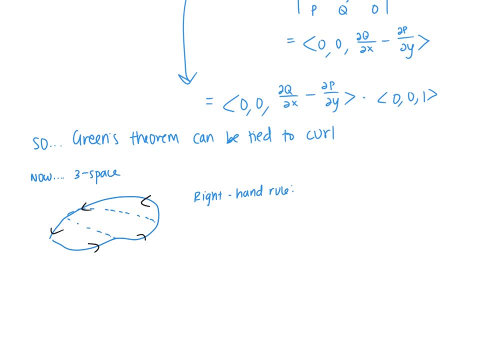 when you use your right hand, the surface has to be on your left. Surface being on your left will give positive orientation. Orientation is either going to be up or down, So we have to figure out: is this going to be oriented upwards or downwards? 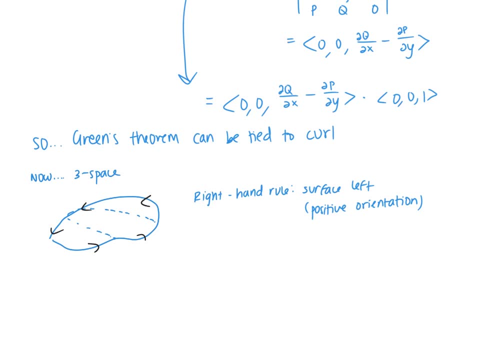 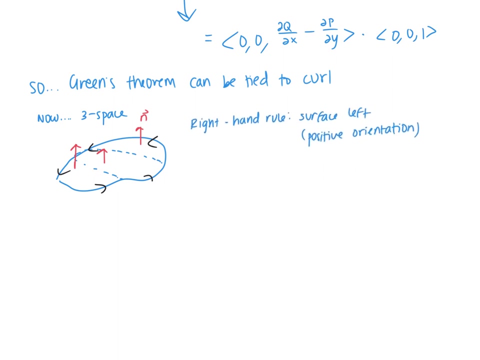 If you picture having your right hand and moving it along the curve following the orientation that it has, that tells you that this is oriented upwards. So we have to figure out what's going to be in the right-hand side. So this relates to Stokes' theorem. 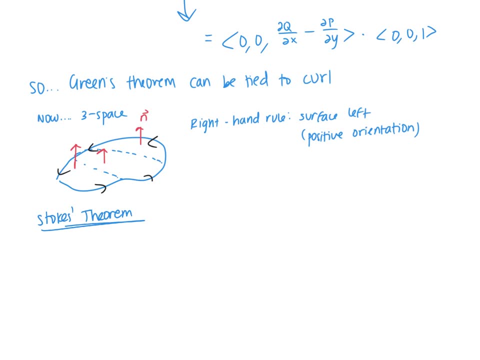 or it leads us to Stokes' theorem. Here's what Stokes' theorem says: Let S be an oriented, piecewise, smooth surface bounded by a curve C with positive orientation. And here's what Stokes' theorem says: The line integral of F, dot dr. 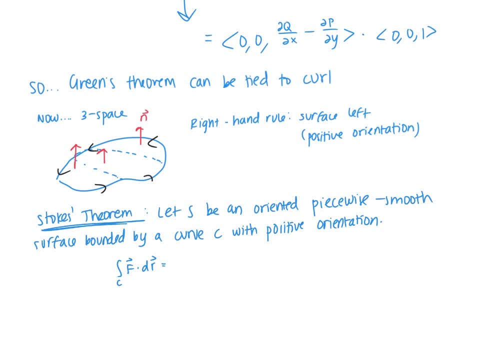 is the line integral of F dot dr can also be calculated as the surface integral of curl of F dot ds. Everything we're going to do today is just related to this theorem. Can I keep going? Is the ds a capital S or a lowercase? 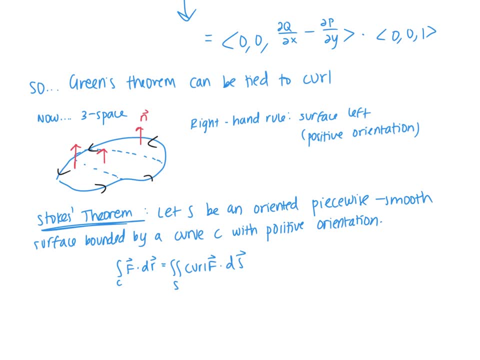 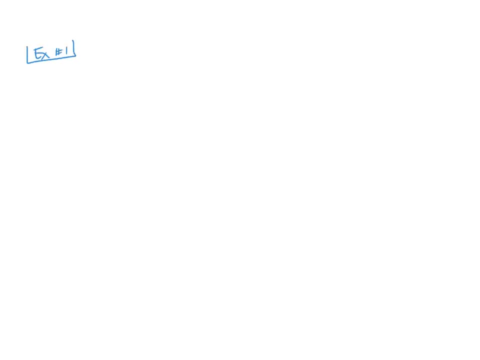 Capital. With a surface integral, it will always be capital. Okay, here's our first example. Let's take F of x, y, z to be x squared and x squared. Four: x y cubed and x y squared. 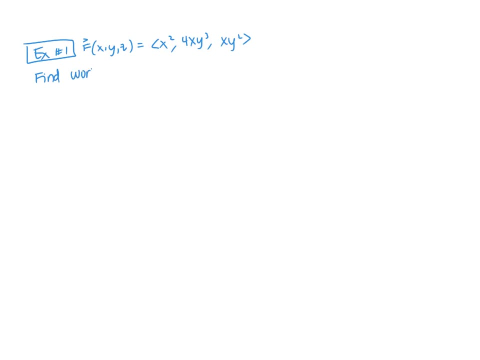 And we are going to find the work done by F on a particle traversing z equals y as shown. So it's not going to be one that is the right answer, but an x squared. So that's my first example, And then I have to find the square root of z. 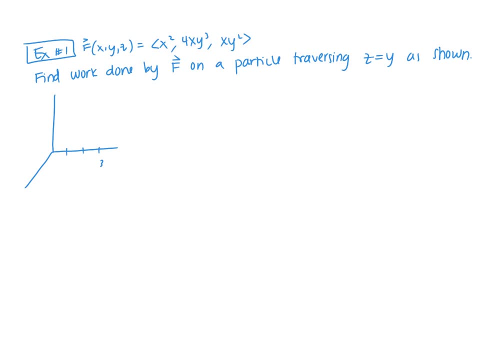 If it's square root of z, I'm going to have to make a square root of z the square root of y. I need to keep writing the square root of y on my x, So I'm going to write it down. I'm going to write the square root of y. 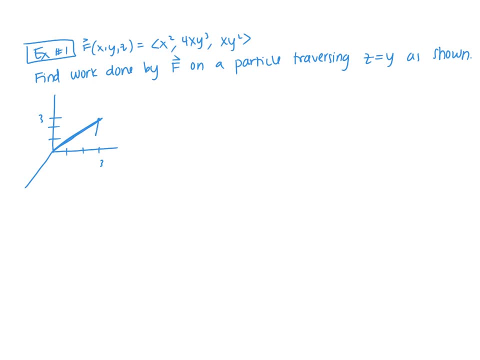 with the exponent of z, And whenever I write something and I it has a miniscule exponent, there's always one left over. So I'm just going to write the square root of z. I'm going to write the square root of y. 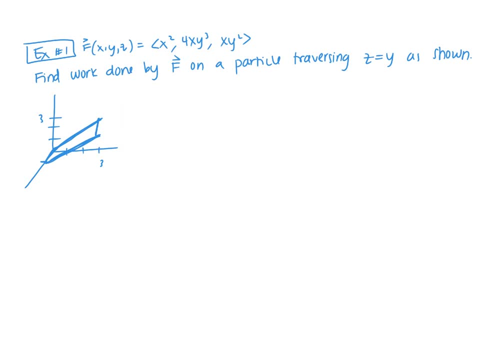 And just follow the way I wrote this, So you don't have to worry about the two. You can do that using your head. Okay, so this is the part of the plane that I'm talking about, and then that's our orientation. 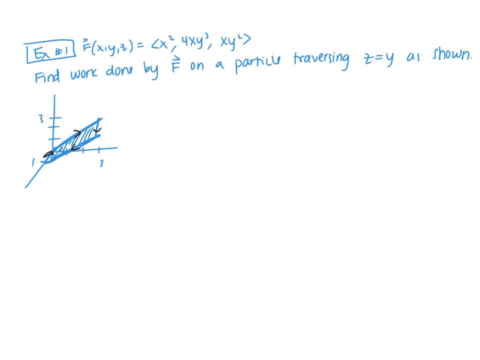 So obviously we know we're going to use Stokes' theorem. Before we talk about why we're going to use Stokes' theorem, I want us to talk about how we would have done this problem 10 minutes ago, before we learned Stokes' theorem. 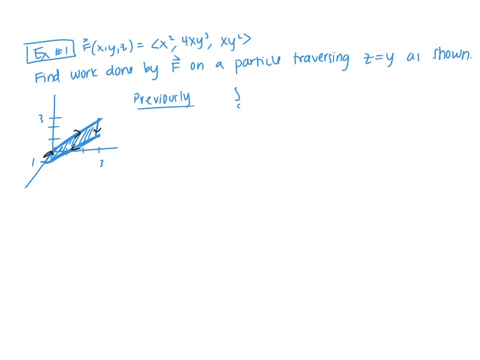 So first of all, with work, it's going to be the line integral of f, dot, dr. So for any line integral, first option is you can use Green's theorem If your curve is on the xy plane. So in our case that doesn't apply. 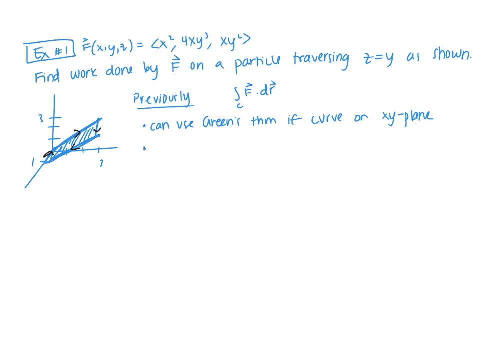 Our curve is not on the xy plane. So instead, what we would have had to do is we would have had to parameterize all four lines and set up four separate line integrals, So we would have had the line integral of the first line. 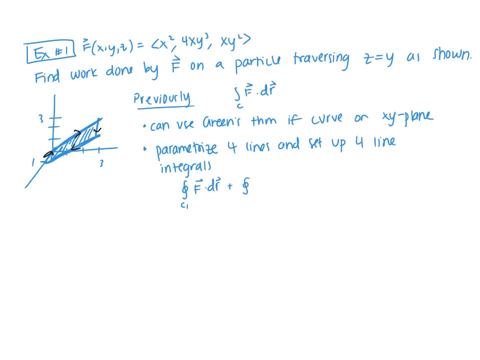 Then we would have had line integral of the second one, so on and so forth up until the fourth one. So obviously we don't want to do four separate line integrals. We don't want to have to parameterize all four of those lines. 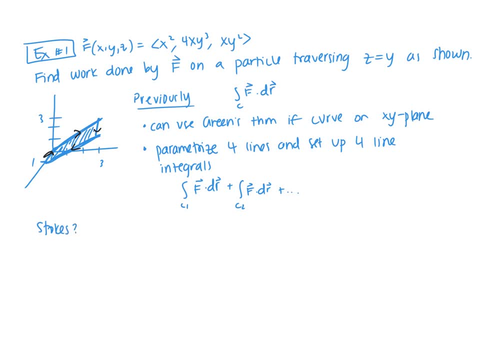 So the question is: can we use Stokes' theorem? Okay, So first of all, we're going to have to parameterize all four of those lines. So first of all, the surface has to be smooth, which we have. 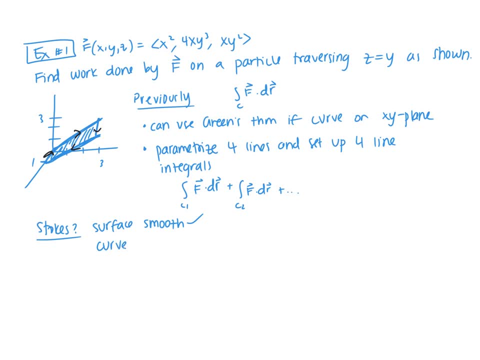 Then we have to have a curve with positive orientation. So we have to figure out what positive orientation means in this case. Again, you're using the right-hand rule, So picture your right. You're using your right hand, traveling around the curve and you need to make sure that. 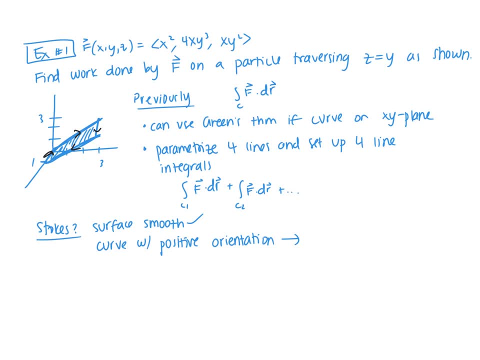 you keep the curve to your left. It's going to be the opposite of the first example we looked at, where this will be our positive orientation. So, yes, we can make that happen if n is down. If we remember from the last set of notes, finding n when our surface is down is going to be positive orientation. 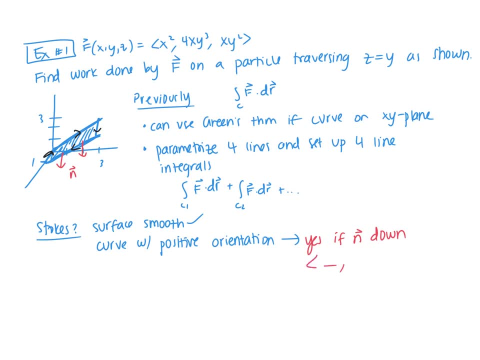 So we're going to find the n component down. We're going to find the n component when our surface is oriented downward. If you remember, there were three components. Last one means the last down, means that the last component is negative one. 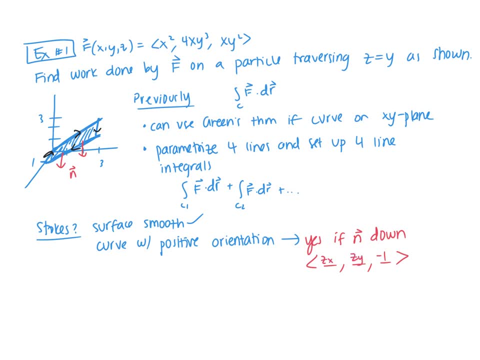 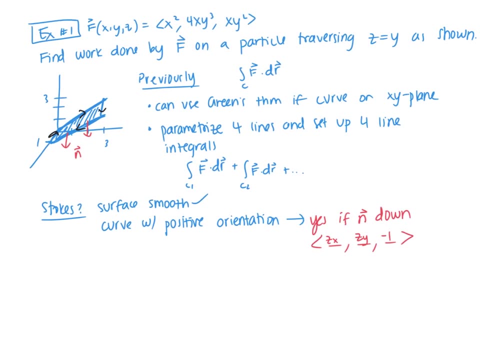 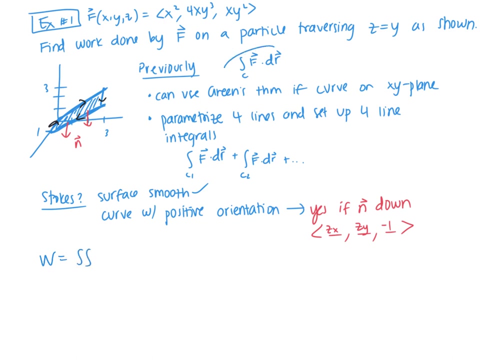 And then we have positive z of x, positive z of y. So that's how we're going to find our n eventually. We're not going to do it yet. Okay, So our work then, instead of using this line integral. 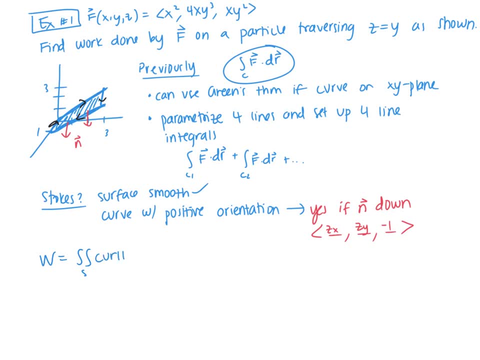 We can calculate it as surface integral of curl of f, dot, ds. So let's find our curl of f. So it's the gradient which is the partial with respect to x, partial with respect to y and partial with respect to z, of f. 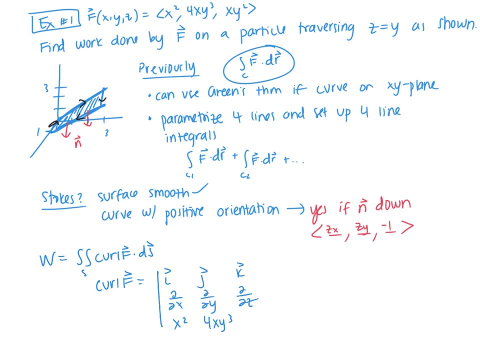 And f is x squared, 4xy cubed, x- y squared. So if we find the i component, we get 2xy minus 0, which gives us 2xy. For the j component, we get y squared minus 0, but then we have to flip the sign. 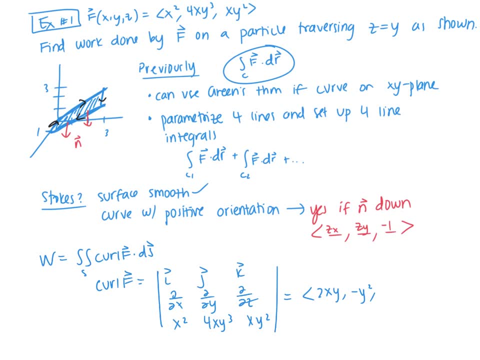 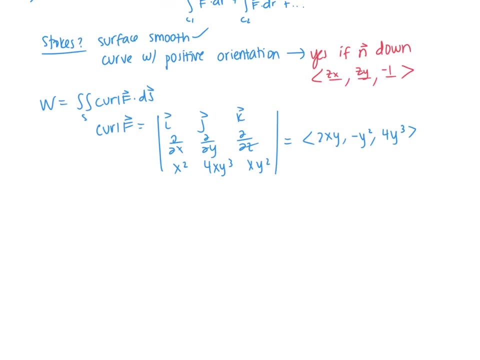 And for the k component we get 4y cubed minus 0, or 4y cubed. So then this is going to become the double integral over the region r of that curl of f, so that 2xy negative y squared, 4y cubed dotted with n. 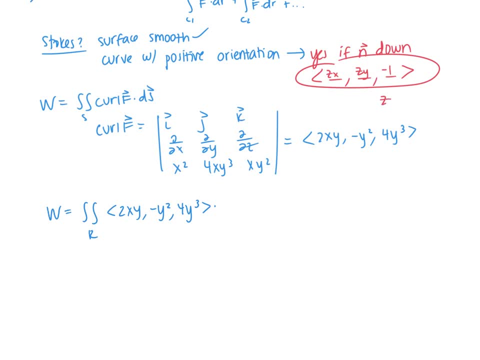 Dotted with n, Keeping in mind that our surface is z Equals y, So the partial with respect to x is going to be 0.. Partial with respect to y is 1.. And then we have a negative 1.. So then that would become negative y squared minus 4y cubed. 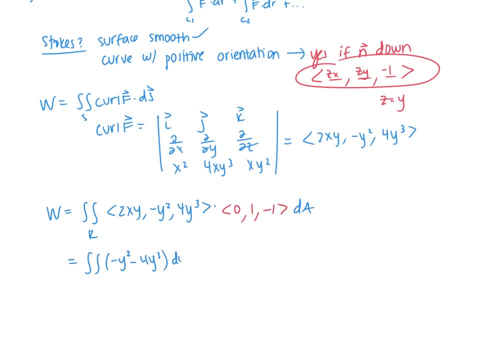 Our region, thankfully, is rectangular, So I'm going to integrate. I'm going to integrate with respect to y first, and then x. y goes from 0 to 3, and x goes from 0 to 1.. And if you trust me, I will tell you: you get an answer of negative 90.. 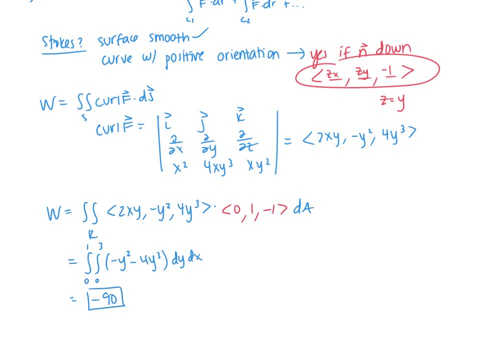 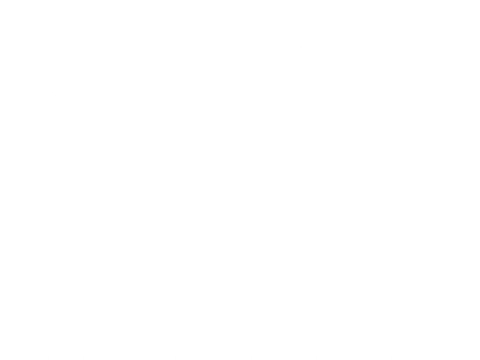 Thank you Questions. before we look at another one. Okay, Let's try another one. Evaluate the line integral of f dot dr. where f of x, y, z is equal to negative, y squared i plus xj, add z squared k. 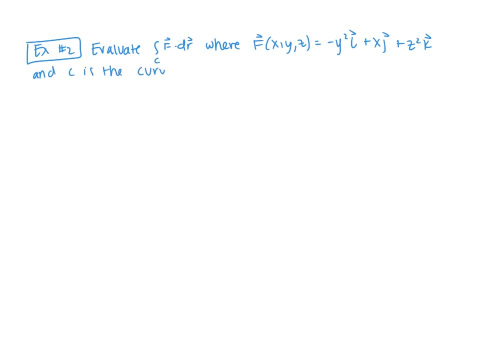 And c is the curve of intersection. So if we have a line integral of y plus z equals 2, and x squared plus y squared equals 1,, we are going to orient c to be counterclockwise when viewed from above. The first thing we're going to have to do is we're going to have to draw a picture to figure out what this curve is. 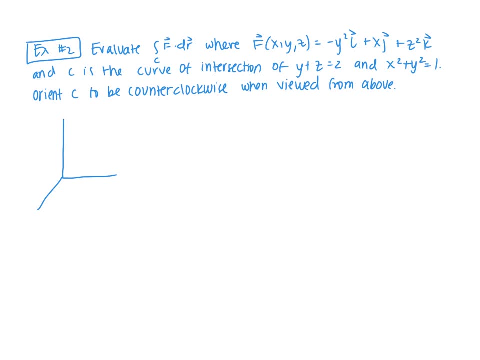 Okay, x squared plus y squared equals 1.. We should be able to tell it's going to be a cylinder, and then y plus z equals 2 is a plane. So we have our cylinder coming up, but then it gets cut off by this plane. 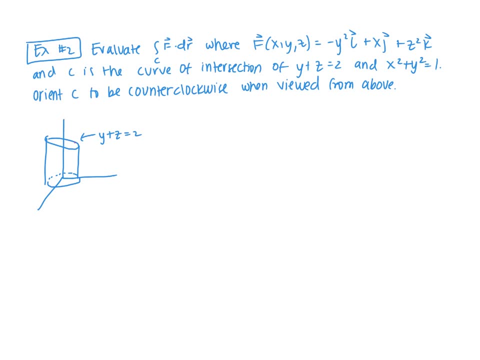 Okay, so our curve C, then, is right here. So that is our curve C, And we are told that it's oriented counterclockwise when viewed from above. So that would be here and there. Okay. so here's the thought process that we need to go through. 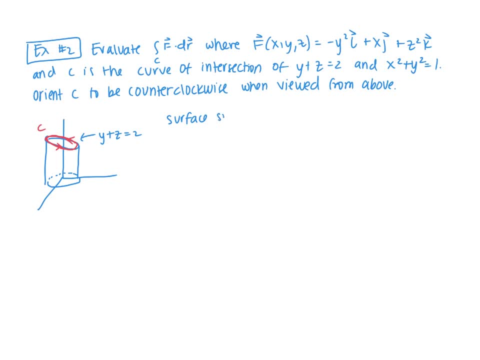 To use Stokes. do we have a smooth surface? Yes, we do. Do we have a curve? Do we have a curve with positive orientation? Well, using the right-hand rule, figuring out where our n would be, our n would be going up. 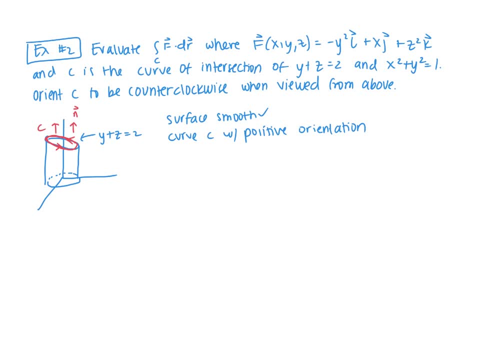 So that's the positive orientation that we're going to use. Okay, so then it's going to be negative z of x, negative z of y and positive 1. Eventually, when we get to the point, we're going to have a positive orientation. 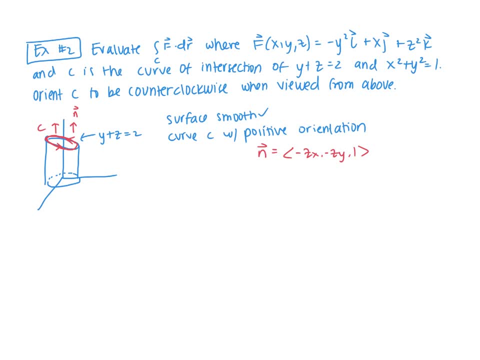 of calculating that. Okay, so both of those are met. That tells us we can use Stokes' theorem. So that's what we're going to do. Again, you're going to start by finding the curl of F, Crossing the gradient with F. 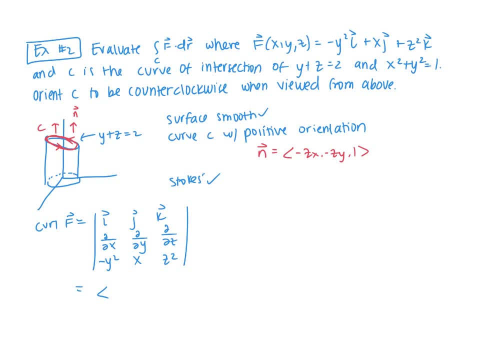 Okay so, finding the I component, we get 0, subtract 0.. Finding the J component: we get 0, subtract 0. again, Finding the K component, we get 1 minus negative 2y or 1 plus 2y. 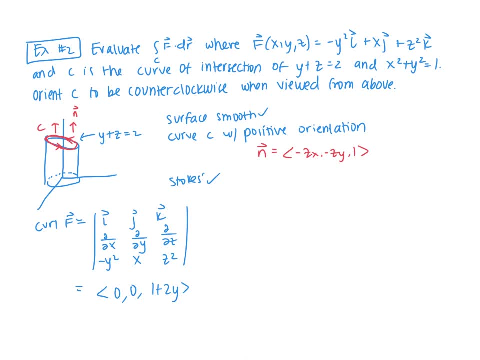 Finding our N. Our N is going to be based off of our Z surface. So if we take that y plus z equals 2, that tells us that z equals 2 minus y, So our N then will be 0,, 1, 1.. 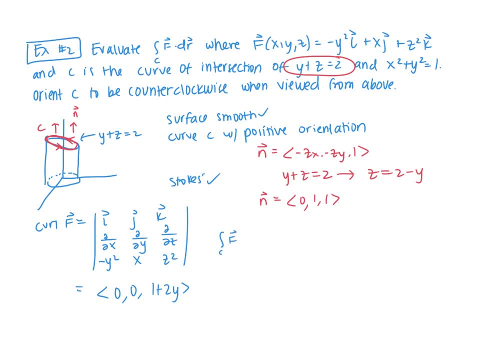 So now we're ready to evaluate. We have that line integral of F dot dr. That's what we want to evaluate. So this is going to become a double integral of curl of F, So 0, 0, 1 plus 2y dotted with 0, 1, 1.. 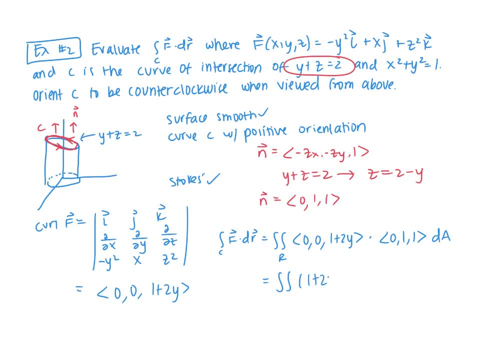 This is going to become double integral of 1 plus 2y. So then, figuring out where our region R is, Our region R is the region in the xy plane, So it's going to be that circle which tells us we should probably convert to polar. 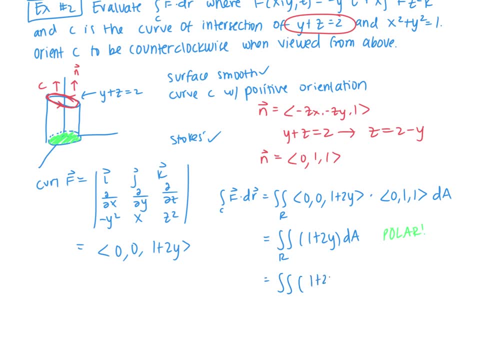 So this becomes 1 plus 2r sine of theta r, dr, d. theta R goes from 0 to 1.. Theta goes from 0 to 2 pi Okay, And you all have calculated so many doubles, So we're going to do a couple integrals at this point. 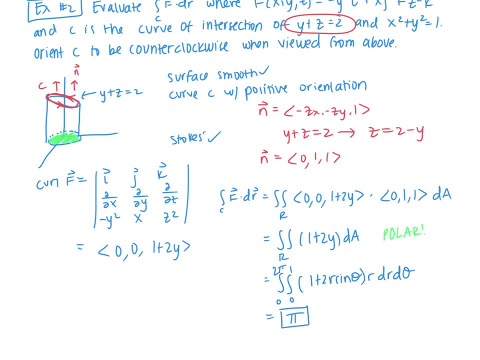 We're not actually going to do the calculation. I'm just going to tell you that it ends up being pi. Okay, Questions before we keep going. Okay, I don't think that Stokes' theory, Stokes' theorem, is incredibly complicated. What is most difficult, in my opinion, is: you can tell from Stokes' theorem. 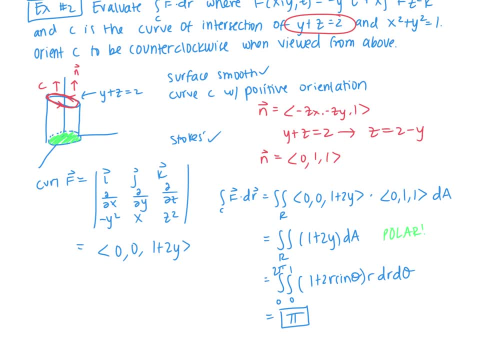 it equates a line integral with a surface integral. So it is going to be up to you to determine when it is more appropriate to use a line integral versus a surface integral. Sometimes it's going to be easier to use Stokes' theorem. Sometimes it'll be easier just to treat it like a normal line integral. 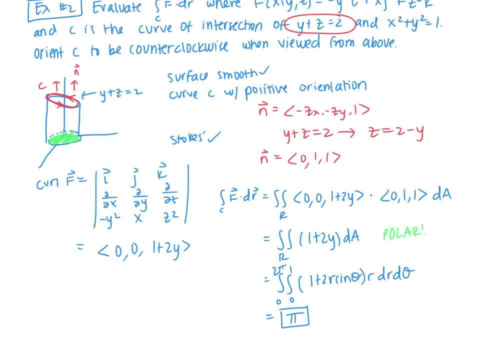 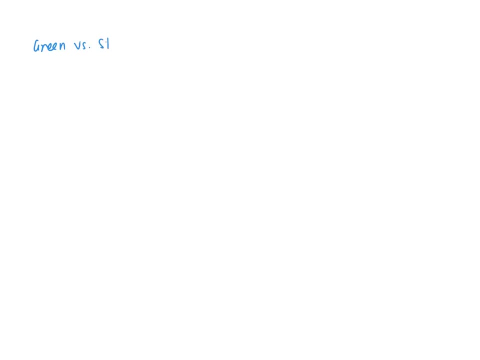 So we have two examples we're going to look at and then we will be done. Okay, So Green's theorem versus Stokes' theorem. Green's theorem takes that closed integral line integral of f, dot, dr and it turns us into a double integral of partial of q with respect to x. 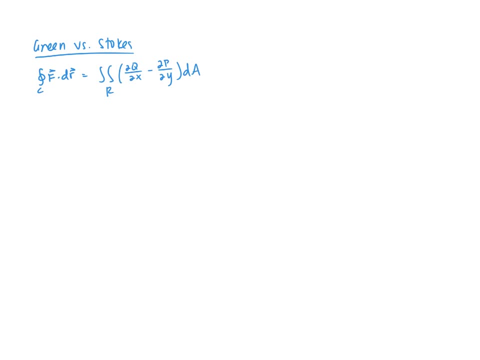 subtract partial of p with respect to y, dA. Okay, So that's Okay. So that's Green's theorem. that is just a special case of Stokes' theorem. That's what we talked about on the first page. So Green's theorem is just a special case of Stokes' theorem. 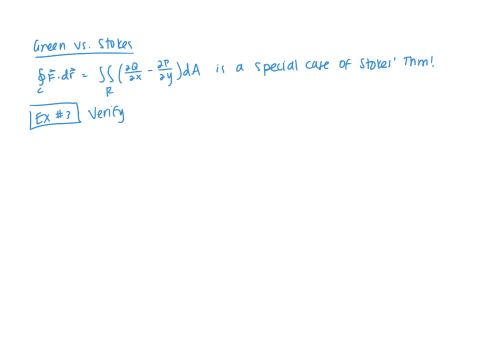 Okay, Third example: We are going to verify Stokes' theorem. for f of x, y, z is equal to 2z, 3x, 5y. where s is the surface, z equals 4 minus x squared, minus y squared. 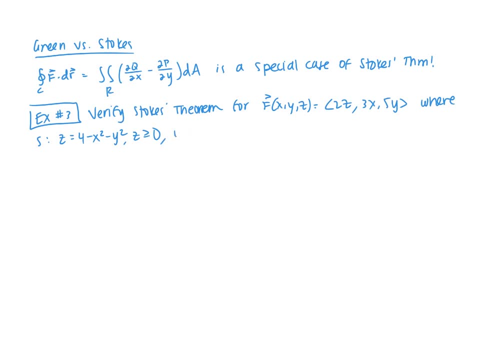 and z is greater than or equal to 0.. With upward orientation, And c is the curve: x squared plus y squared equals 4.. On the x- y plane With positive orientation, so, starting with a picture, z equals 4 minus x squared, minus y squared. 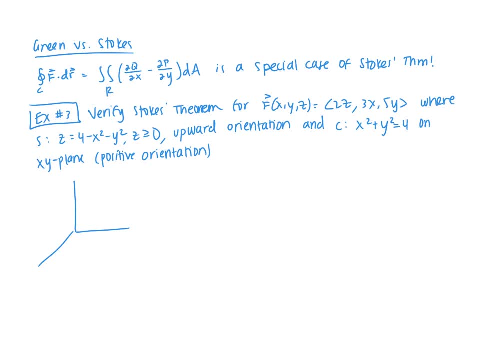 it's a paraboloid opening down. it has a z intercept at 2- nope, I lied at 4. this is what we're looking at. this upper part right here is our surface and it has upward orientation. and then we are also told that our z squared minus x squared. 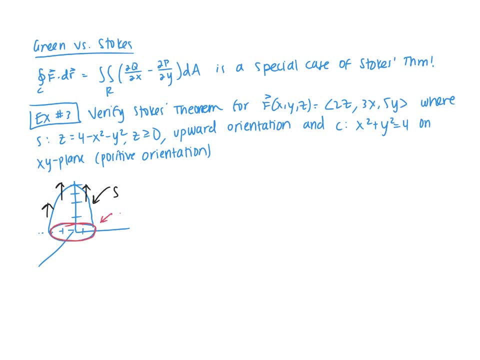 is our z intercept. at 2, our curve is this circle: x squared plus y squared equals 4, with positive orientation. So positive orientation meaning that using our right hand rule: when we put our right hand up, the surface is going to be on our left. 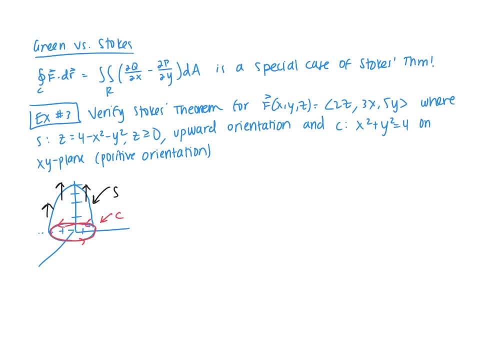 And okay. so first thing we are going to do is we are going to calculate the line integral. So to do that, we are going to have to orient that curve, that red curve. It's a circle. so that gives us 2 cosine of t, 2 sine of t. 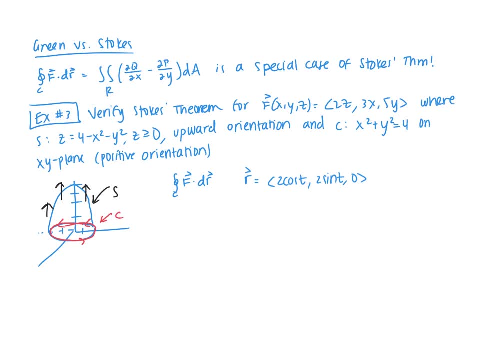 That gives us 2 cosine of t. That gives us 2 sine of t And 0.. So that's going to give us the integral of f of r. So we're going to have to take r and plug it into f. 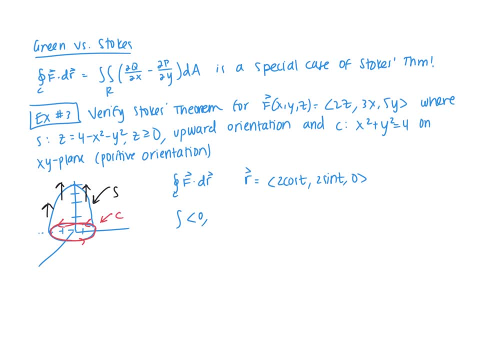 So 2z or 2 times 0, is 0.. 3 times x, so 3 times 2 cosine t gives us 6 cosine t, And then 5 times x. so 3 times 2 cosine t gives us 6 cosine t. 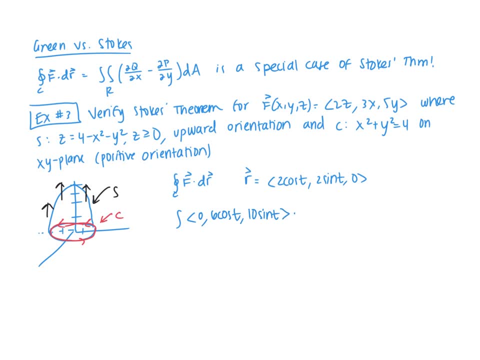 And then 5 times y will give us 10 sine of t. And then, if you remember, we dot that with r, prime of t, which is going to give us negative 2 sine of t, 2 cosine of t and 0.. 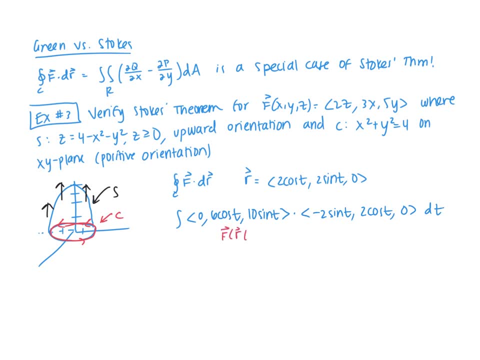 So again, this first one is just f of r And the second one is r prime of t. It's one of the first ways we learn to calculate a line integral. When we multiply that out, we end up getting 12 cosine squared of t- dt. 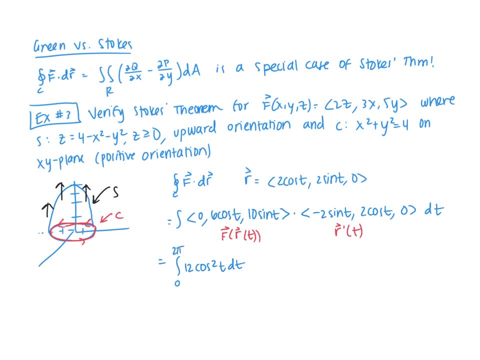 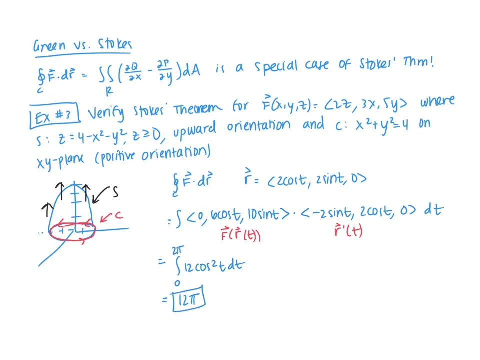 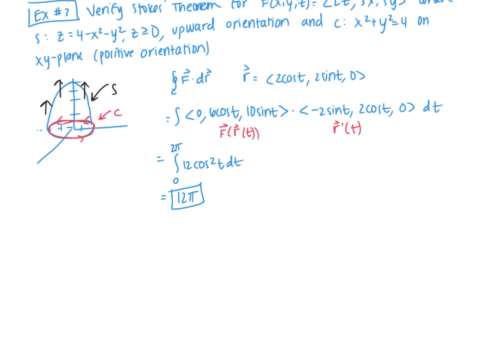 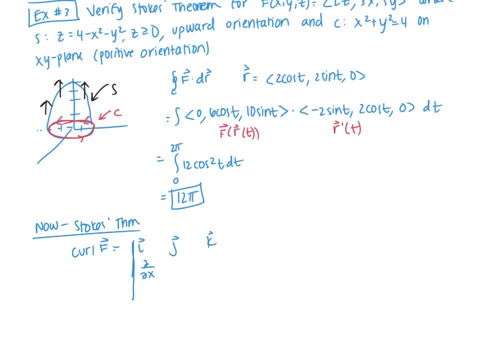 so our f was 2z, 3x and 5y. so we get 5 subtract 3, which is just 5, and then we get 0 subtract 2, but change the sign. then we get 3 minus 0. so then we said that s has upward orientation. 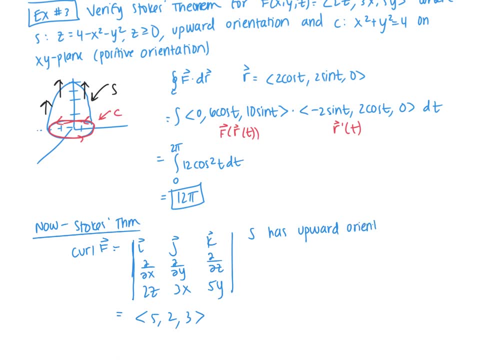 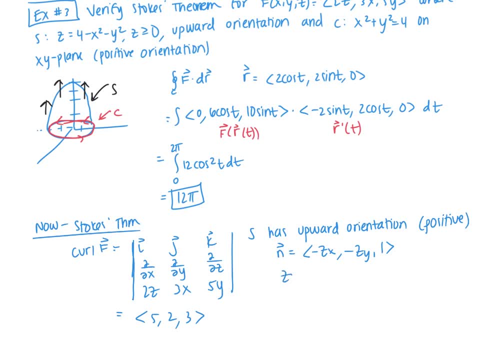 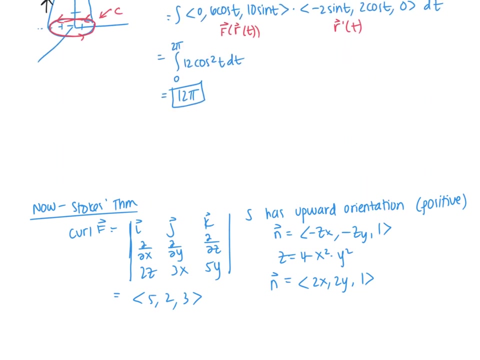 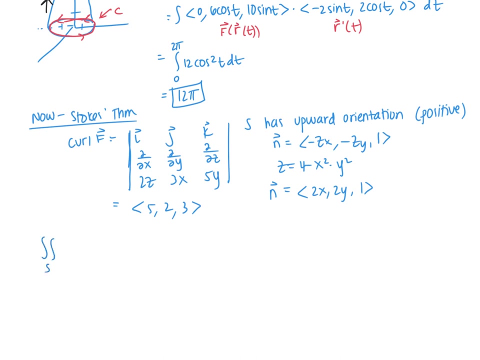 so so, so so, and z is that 4 minus x squared minus y squared, so we're going to get 2x comma 2y comma 1. so then if we want the surface integral of curl of f dot ds, it's going to become the double integral. 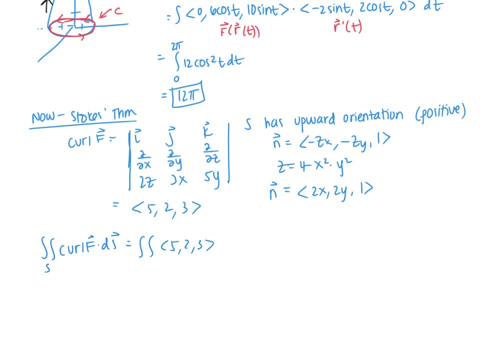 so this is 그걸's of curl of f, so 5, 2, 3, dotted with n, so 2x, 2y, d, by which, which, which becomes 10x, add 4y, d, by which becomes 10x, add 4y, add 3, d, by. 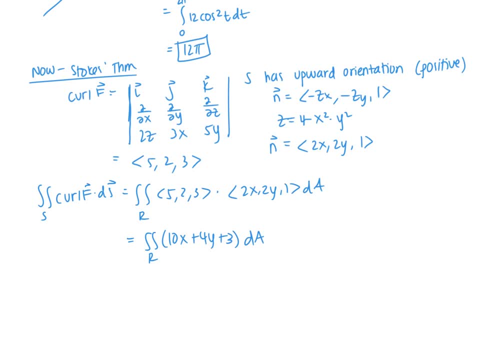 r is just that circle in the xy plane, So we're going to want to convert to polar. So this will be 10r cosine, theta plus 4r sine of theta, Add 3r. dr d theta Circle has a radius from 0 to 2, and theta goes from 0 to 2 pi. 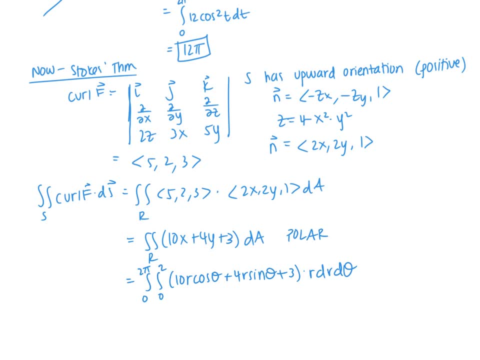 And believe it or not, this would give us an answer of 12 pi. So I would argue, in this case the line integral was significantly quicker, And if we would have recognized that I mean we had to do both, because that's what the problem was. 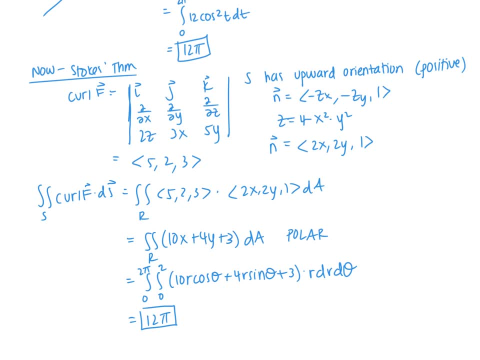 That's what the problem asked us. But if we would recognize that in the homework that it would be easier to do the line integral, it's going to be a lot shorter. We have one last example to do Questions before the last example. 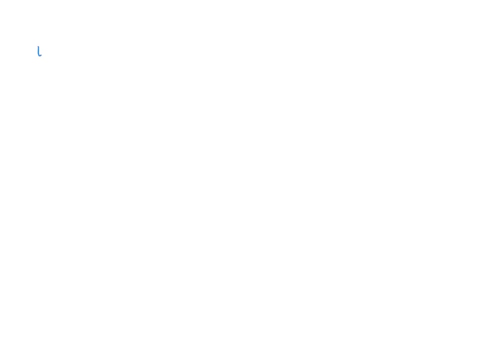 Okay, This last example we are specifically doing so that we can decide what is going to be quicker: a surface integral or a line integral. We are calculating the surface integral of curl of f, dot, ds. f is xz comma, yz comma xy. 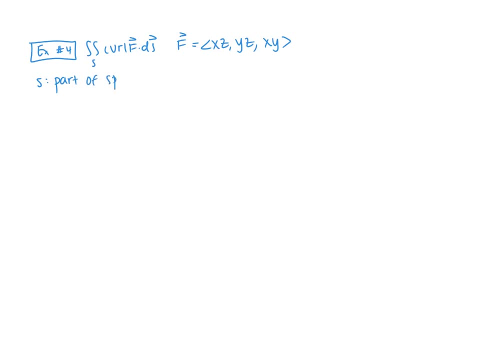 s is the part of the sphere. x squared plus y squared plus z squared equals 4.. That lies inside x squared plus y squared equals 1., And above the xy plane. Okay, Okay, So Let's draw ourselves a picture. 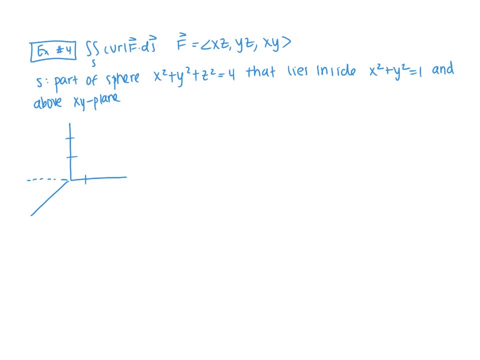 Okay. So if we're above the xy plane, then we're only looking at a hemisphere, We have that part of the hemisphere, But then we have x squared plus y squared equals 1.. So we have to figure out what our s is. 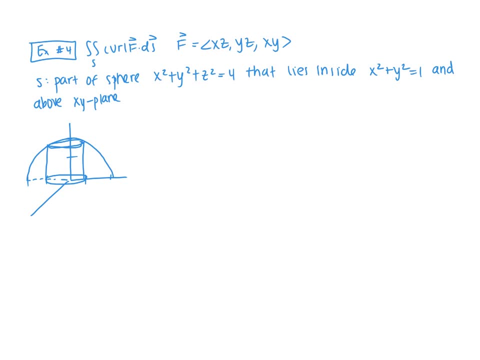 s is the part of the sphere that lies inside the cylinder and above the xy plane. So s is going to be this stuff right here And we're going to do a little bit of math for this. Okay, So if we try to calculate the surface integral- this is an oriented surface- we would have to find n. 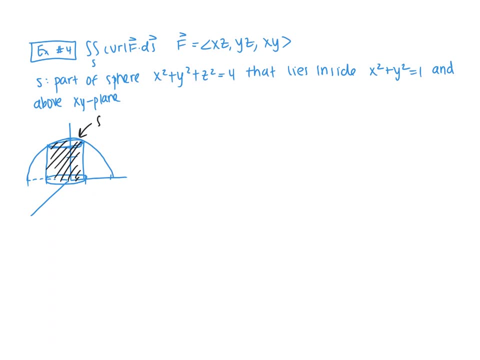 The problem with finding n is we do not have an easy equation for z. So if we wanted to find n, we would have to use this equation, And we would have to find z, And we would have to use this equation, And we would have to use this equation. 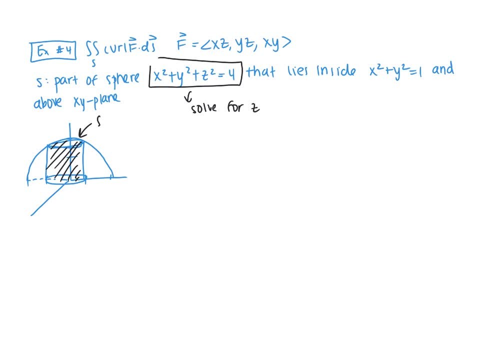 And we would have to use this equation, have to solve for Z to find the vector for our orientation. We don't want to do that. that's not going to be efficient at all. So instead of calculating this as a surface integral, we're going to calculate it as a line integral. This is: 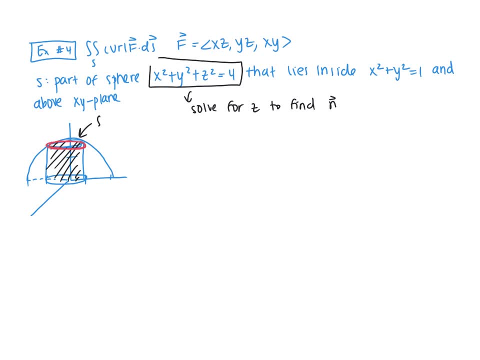 our C. It's the intersection of our two surfaces, So we're going to calculate this as a line integral. instead To do that, we're going to need to find C. So we start with: X squared plus Y squared plus Z squared equals 4.. 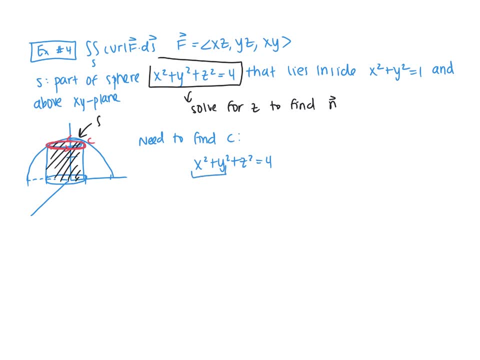 We also know that from our other equation, though, X squared plus Y squared equals 1. Substituting that in it gives us Z squared equals 3. So we're looking at the circle: X squared plus Y squared equals 1, positioned at Z equals root 3.. 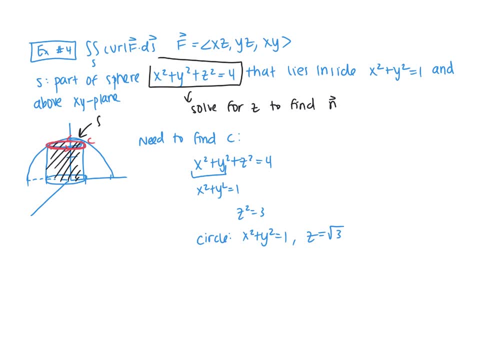 So we are going to treat this as a line integral. Our R of T, based off of that circle that we just found, is cosine of T, comma sine of T, comma root 3, which means our R prime of T then is negative sine of T. So we're going to treat this as a line integral. So 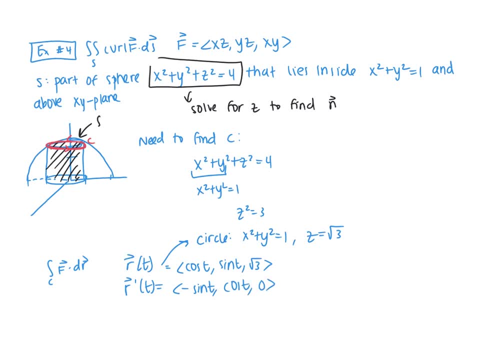 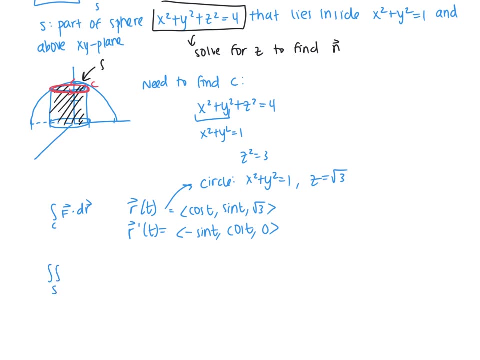 we have cosine of T, cosine of T 0.. So then, surface integral of curl of F dot ds. Stokes' theorem tells us that we can do this as a line integral of F dot dr. Okay, so we're going to take F of R. 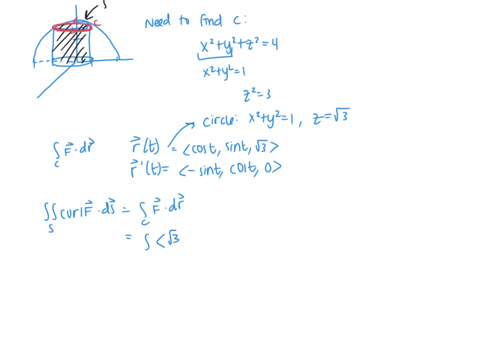 so that's going to be root 3 cosine of T, root 3 sine of T. cosine of T. sine of T dotted with R prime of T. So that's negative sine of T. cosine of T and 0 dt. T is going to go from 0 to 2 pi Alright. so we've got our Y squared plus T, squared plus R times.